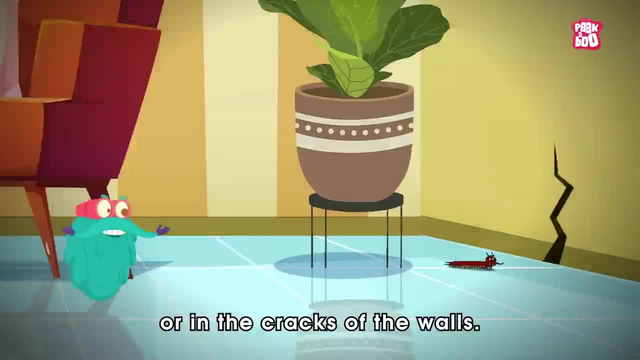 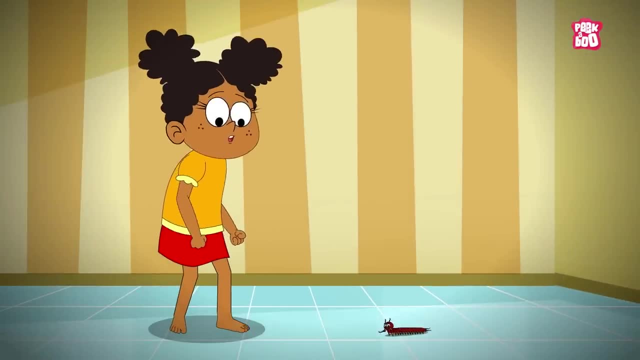 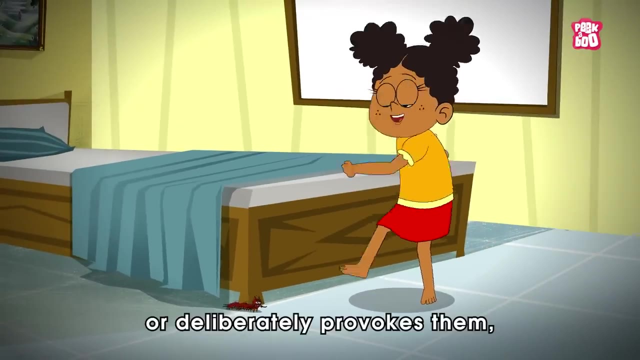 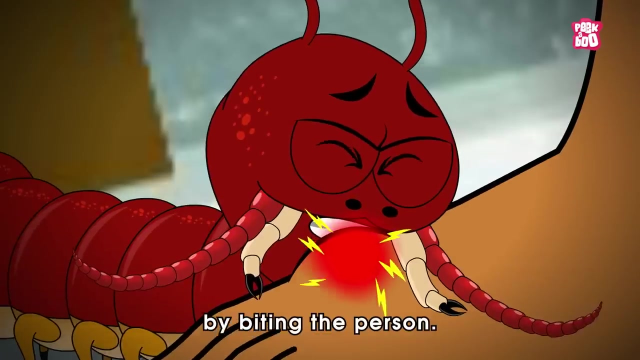 You may find them under the floor or in the cracks of the walls. Mostly, centipedes are not aggressive toward humans and tend to run away from us. However, if someone accidentally steps on them or deliberately provokes them, these creatures won't shy away from defending themselves by biting the person. This can result in two red markings in a V-shape due to the arrangement of the insect's forsythia, Though this bite can be extremely painful, particularly when bitten by larger centipedes that tend to deliver more venom, Fortunately, their venom is generally harmless to humans, causing only mild and temporary effects. 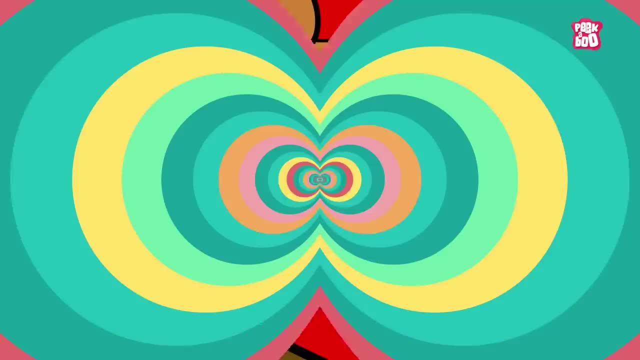 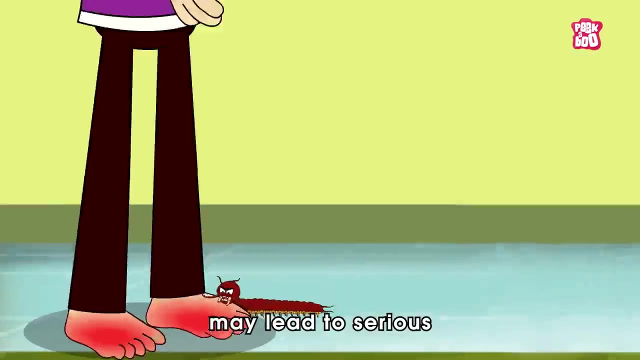 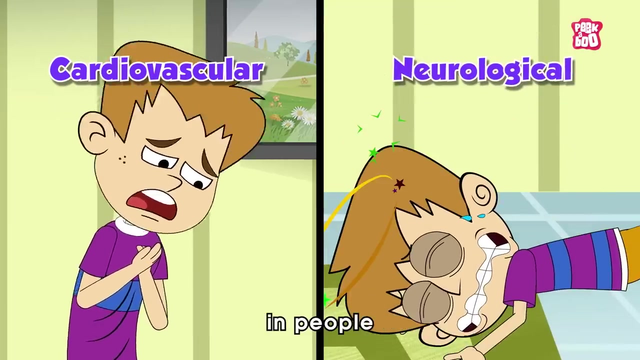 which may go away in a few hours. However, bites from certain species, such as the Scolopendra genus, may lead to serious allergic reactions, as well as cardiovascular and neurological effects in patients Due to the strong chemical composition of their venom. 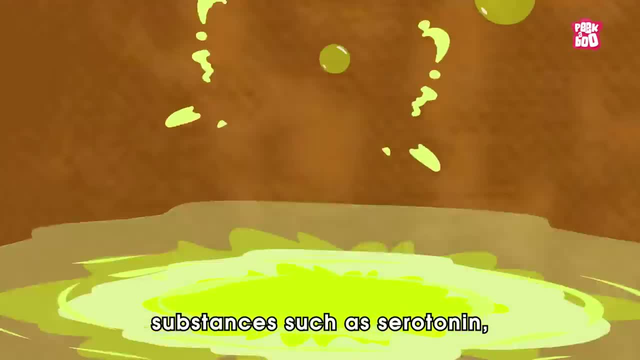 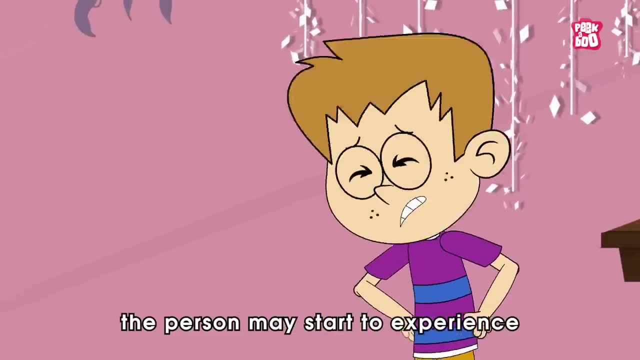 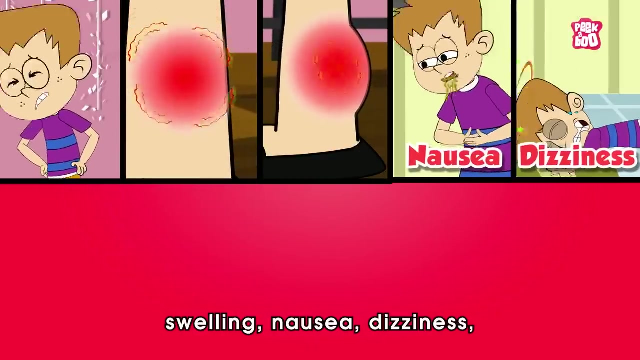 which contains substances such as serotonin, histamine and cardio-depressant toxin S. soon the person may start to experience symptoms such as intense pain radiating from the bite site, swelling, nausea, dizziness, difficulty in breathing, rapid heart rate and even fever and chills. 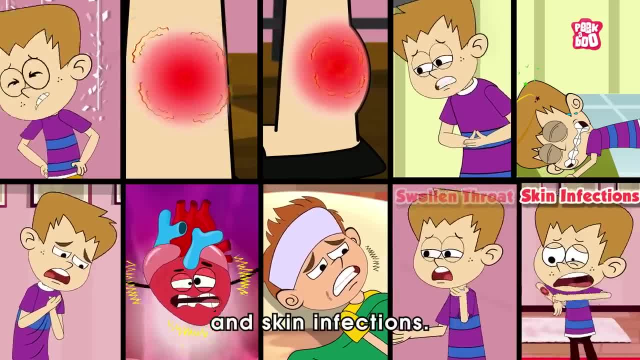 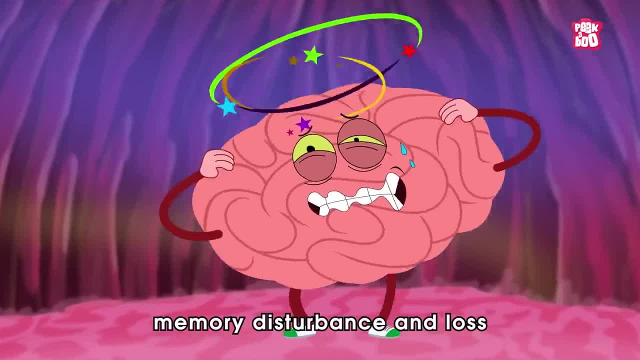 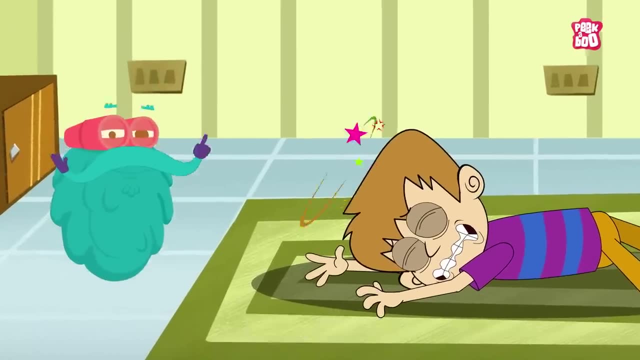 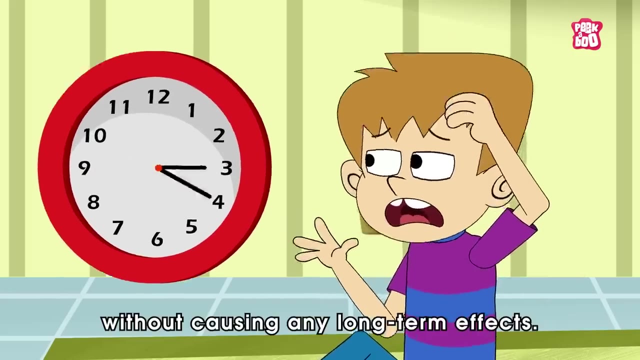 along with a swollen throat. In some extreme cases, the person may even experience memory disturbance and loss of consciousness. Fortunately, these serious conditions rarely occur and for most centipede bites, the symptoms may resolve within a few hours to days without causing any long-term effects. 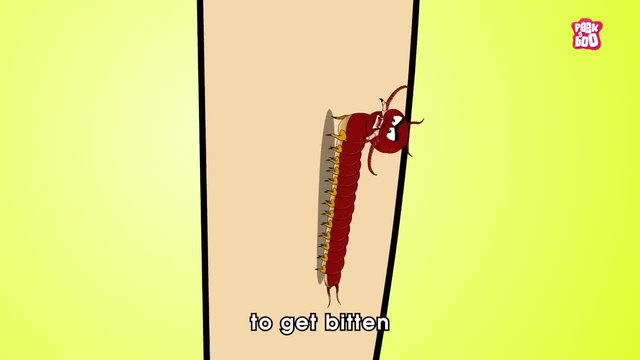 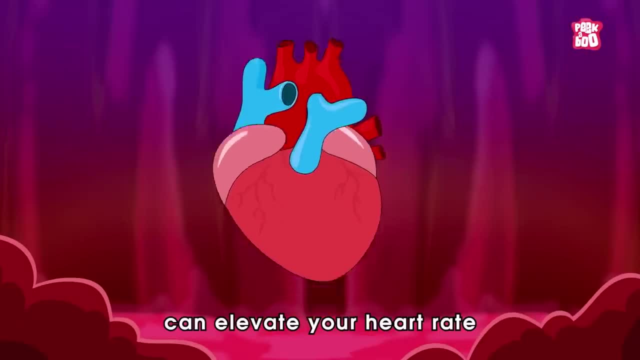 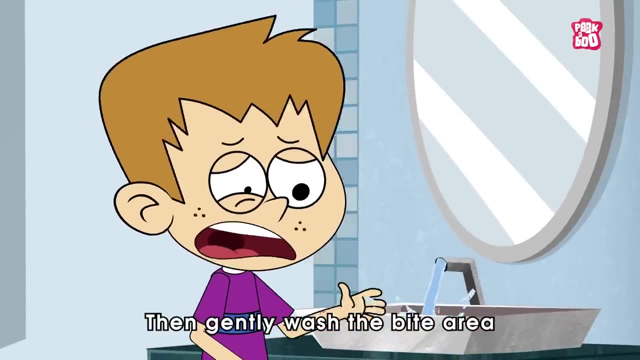 But in case you happen to get bitten by a centipede accidentally, make sure to remain calm, as panicking can elevate your heart rate and increase the spread of venom throughout the body. Then gently wash the bite area with mild soap and water to reduce the risk of infection. 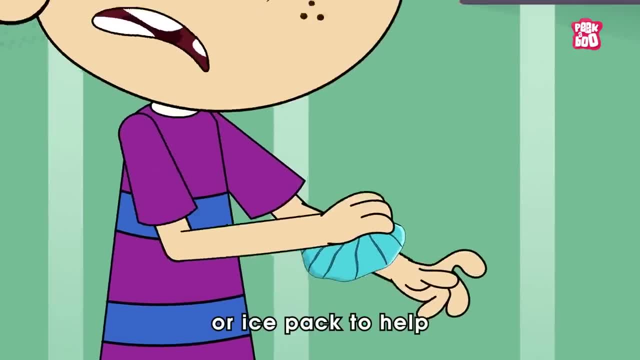 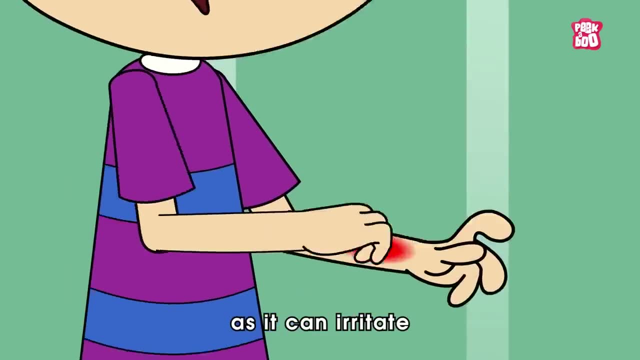 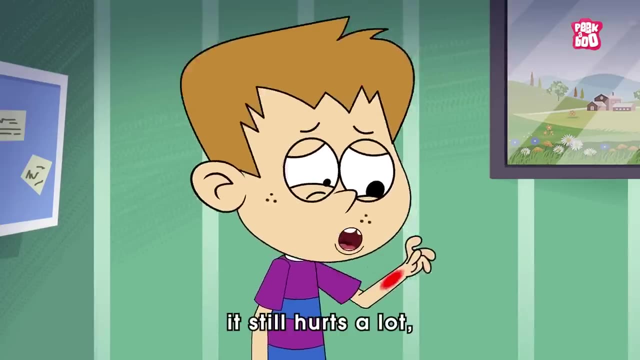 Afterward apply a cold compress or ice pack to help relieve pain and swelling. Also, remember not to scratch the bite, as it can irritate the skin, making it easier for germs to get in In case. even after some time, it still hurts a lot.